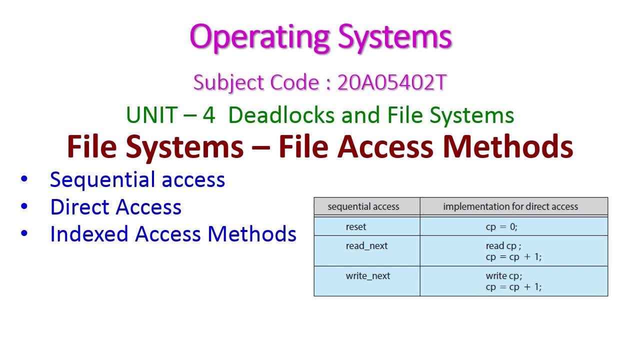 Hello friends, in this operating system class we will see the file access methods, and there are three file access methods. First one is sequential access, direct access and the indexed access methods. Let us see all these things one by one in today's class. 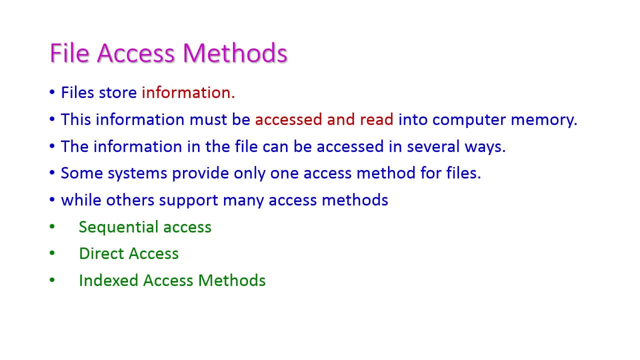 Okay, before that, let us see what is file access method. We know file stores information. This is a file which contains information and this information must be accessed and read into computer memory. Okay, all these files will be stored in the computer memory. Okay, this is computer memory. 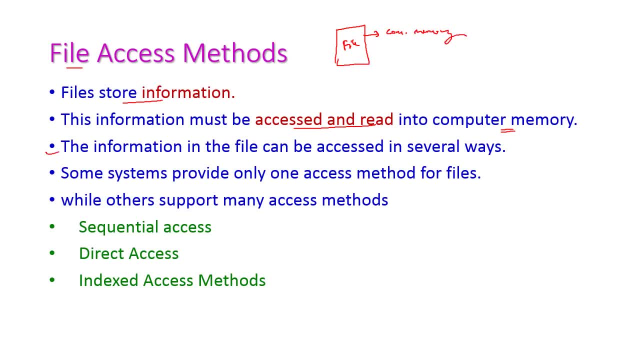 Okay, this information is stored in the computer memory. Okay, this information in the file can be accessed in several ways. Now I want to access this particular file. There are different methods to access this file. Some system provide only one access method and some system supports many access methods. Okay, the different methods are sequential access, direct access and indexed access methods. 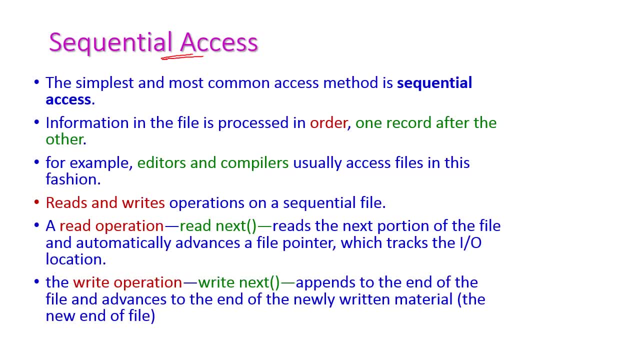 The first one is sequential file access. This is the way to access the file. This is the very simplest and most common access method. Here the information will be stored in order, That is, one record after another record. Okay, for example, this is the sequential file, And in this sequential file the file will be loaded one after another. Okay, one by one, the records will be ordered. This is 01234, like this: 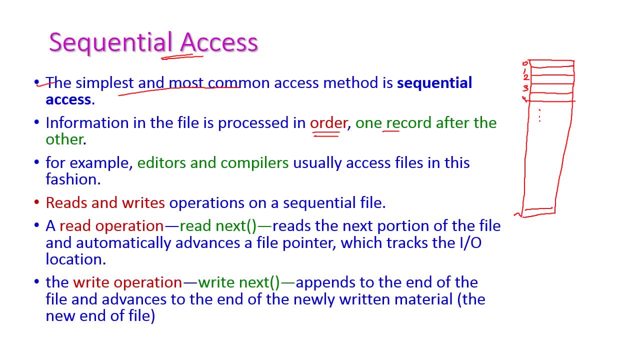 And this is here Okay. n number of records will be stored in this sequential file. For example, the editors and compilers usefully access the files in sequential fashion. Okay, one after another, And the reads and write operations are most common in sequential file. Let us see how these reads and write operations will be taken place. 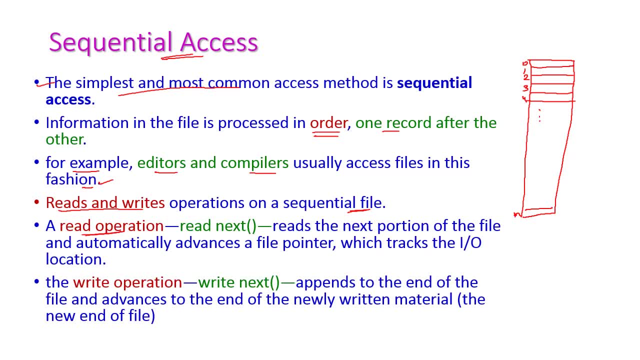 First let us take this read operation. See, once we perform the read operation, the file pointer will always point in the beginning of the file BOM. beginning of the file. Okay, see, once it reads the first record, then it will read automatically Next record that is read next. read next means the file post that is the next portion of file and automatically advances the file pointer. Okay, the file pointer will give us the first record. 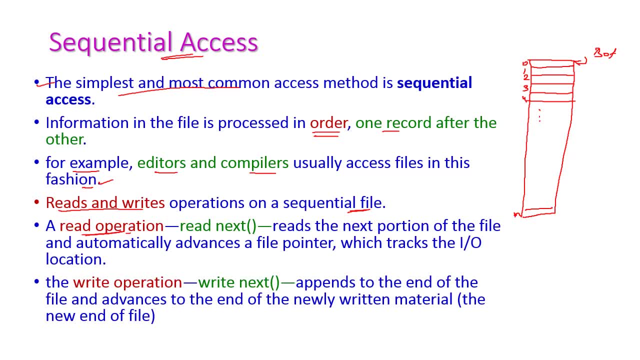 You can see, once we send a file to this file. This is the first record. after the second record that is read full pressем. Next order is automatically read: Nina, Okay, the find point will give us the file pointer after read access. as the pressing of the 너stere first question, we'll give the on gel log points follow up the necmand address panel. 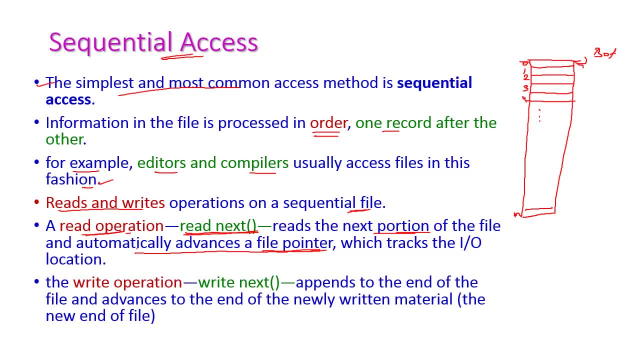 the file pointer will be incremented by 1 automatically. That is read next: Okay, And when come to write operation, the file pointer will automatically come to the end of file: EOF. Okay, End of file. And if any write taken place on the record. 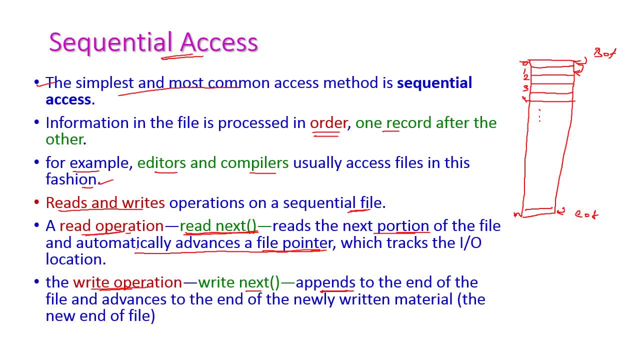 and immediately. that appends to the end of the file Okay, And advances to the end of the file. newly written material, That is, the file pointer, will be incremented into the new end of file location. Okay, This is N plus 1th location. 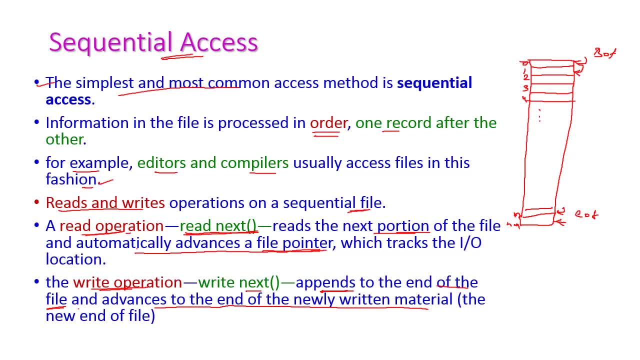 Okay, This is how the sequential operations, that is, read operation and write operations, will be taken place in the sequential file. Okay, Sequential file means all the records will be ordered one after another And the read operation or write operations will be taken place in the sequential manner. 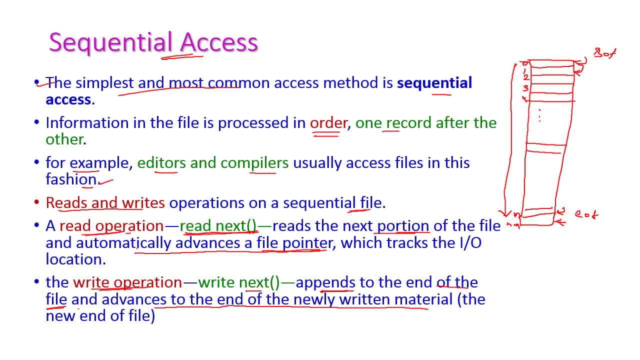 And it is not possible to read the record which is in the middle. Okay, If we want to read only this particular record, this is not possible in this sequential file access. We have to read all those records one by one. Then only we can reach this. 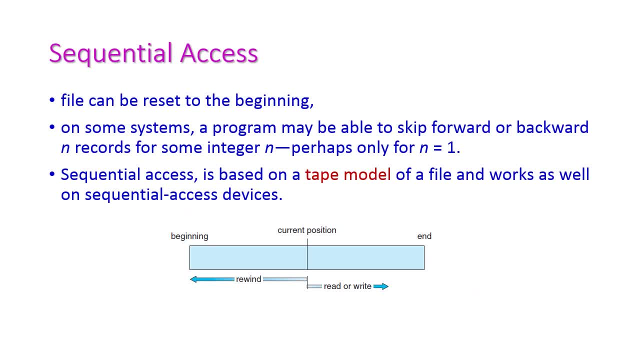 for example, 50th record. Suppose I want to do a read operation. then the file can be reset to the beginning of the file, that is B OF Okay, Suppose the current position is in between. that is middle of the file. 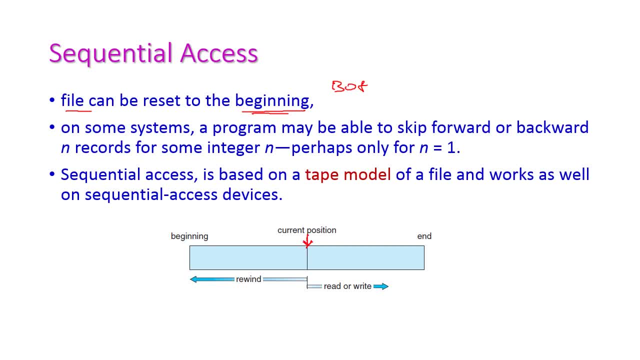 and I want to access some of the record means immediately. the file positions will be rewinded into beginning of the file. Okay, In some system the program may be able to skip forward or backward end records. Okay, For example, if the position is 50,. 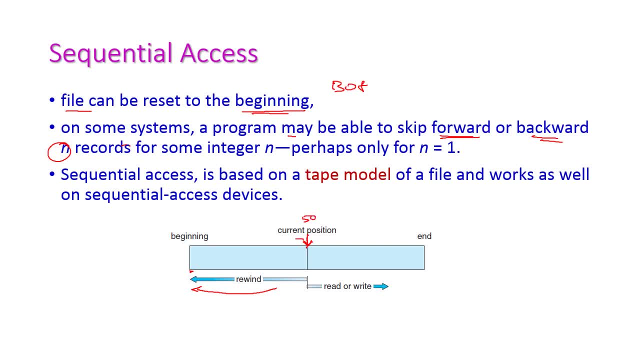 then the rewind will be taken place by end records for some integer, perhaps only for n equal to 1.. That is, if n equal to 1, that is beginning of the file. The file pointer should be rewinded to the beginning of the file. 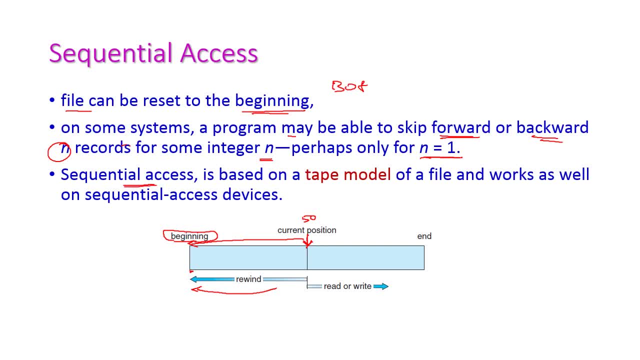 Okay, In sequential access is based on tape model, that is, magnetic tape model. Magnetic tape model magnetic tape device is one of the best example for the sequential access- that is, sequential access of file, and works as well as on sequential access devices. 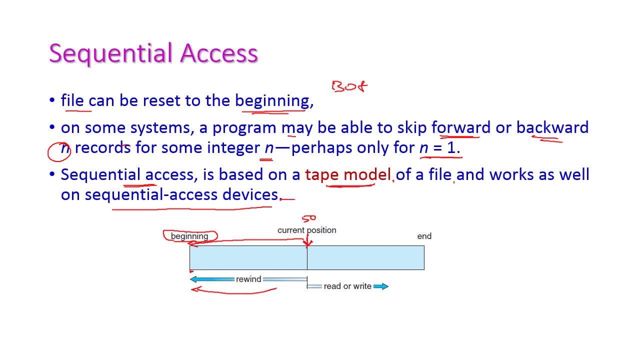 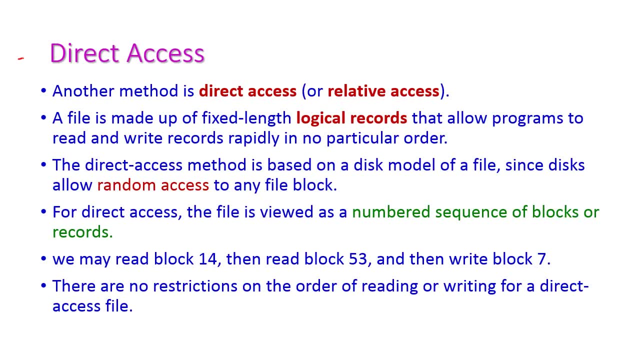 Okay, Magnetic tape model is the best method for sequential file access, Direct access. this is the second model, which is otherwise called as relative access. Okay, Here the file is made up of fixed length of logical records. Right, See here. 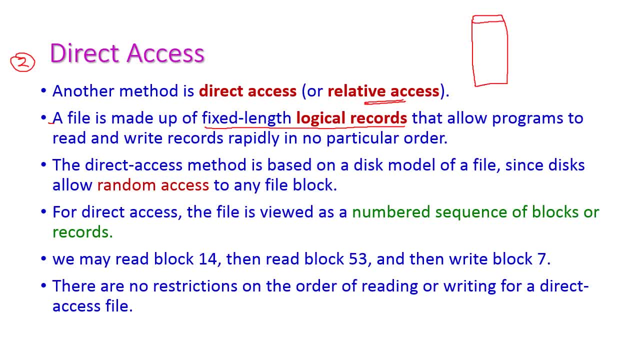 this is the file, and the file contains the collection of records. All the records should have equal size. Okay, Right, Okay. And it allows programs to read and write records rapidly into, in no particular order. This is important, Right, Suppose. 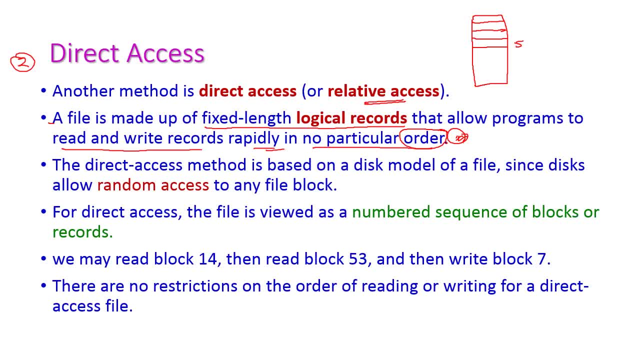 I want to access the fifth record. no need to access the records from the beginning. I can directly set the file pointer to fifth record and I can read the fifth record directly. Okay, The direct access method is based on disk model of your file. 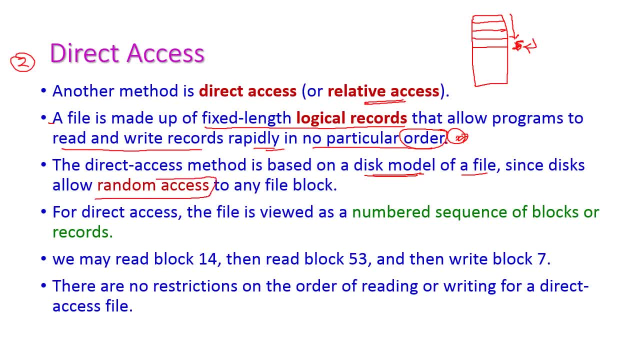 And since disk allows random access to the file blocks- and nowadays all secondary storage devices supports this random access- And for this direct access, the file is viewed as numbered sequence of blocks or records. Okay, So we have to give unique number for all the blocks or all the records. 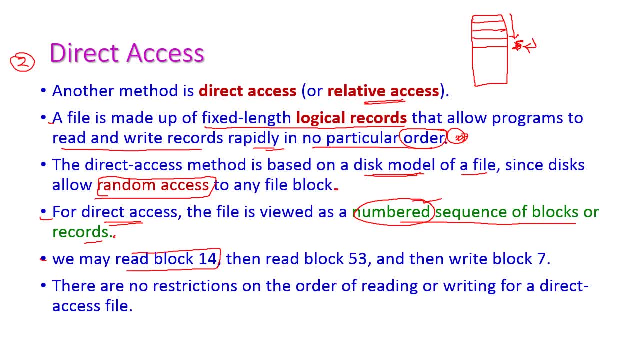 Okay, So that we can read block 14 and we can read block 53.. Okay, There is no restriction to read all the records sequentially. Which record we want, we can directly move to file pointer that location, Then we can directly read that particular record. 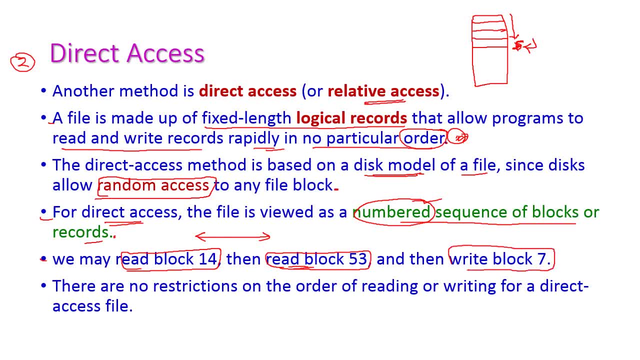 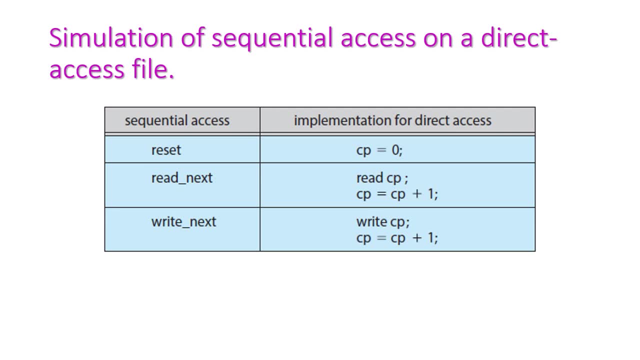 Then immediately we can write block 7.. Okay, This is also possible here. So there is no restriction on the order of reading or writing of direct access file. Next let us see the simulation of sequential access on the direct access file. 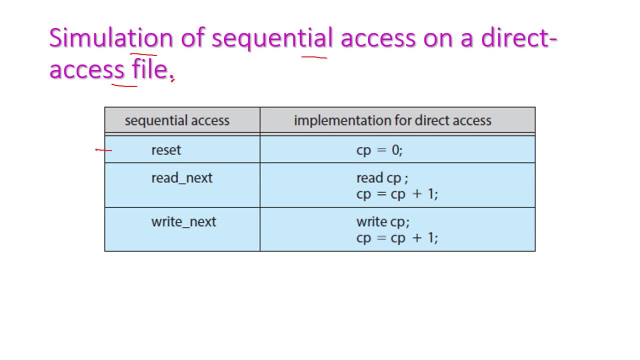 Okay, The first is the sequential access. The reset command is used to move the file pointer into beginning of the file. Okay, Here the current position equal to 0.. When come to direct access, we need to set the current position, which is equal to 0.. 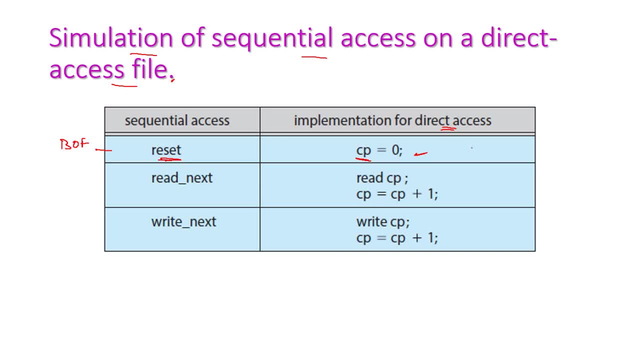 So this will set the current pointer into beginning of the file, Right To read the next record. here in the sequential access we can use read next. But when come to direct access the current position will be incremented by 1 to read the next record. 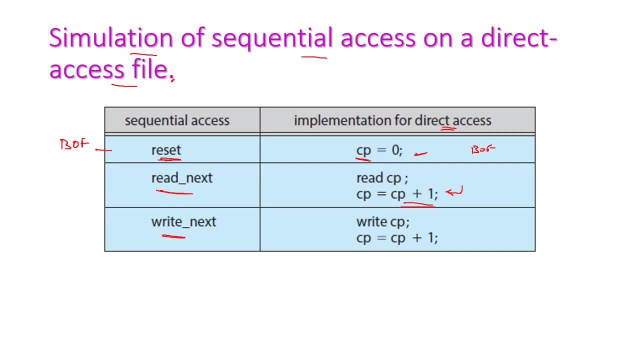 Okay When come to write. to write the next record here in the sequential access we can use write next command. When come to direct access, the current position will be incremented by 1.. Okay For writing. also Indexed access method. 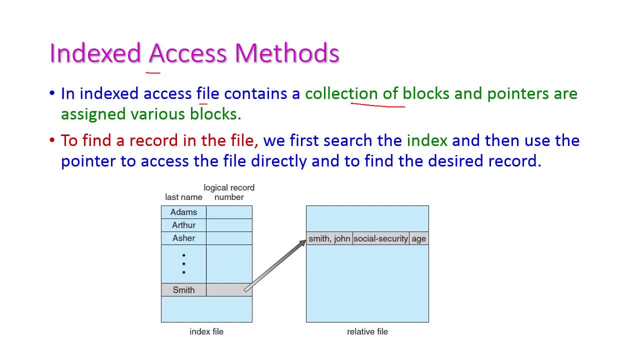 In this file, which contains a collection of blocks of records, and pointers are assigned to various blocks. Okay, By using this pointer we can access the corresponding record. Okay, To find the record in the file, first we have to search the index and then use this pointer to access the file directly and to find the desired record. 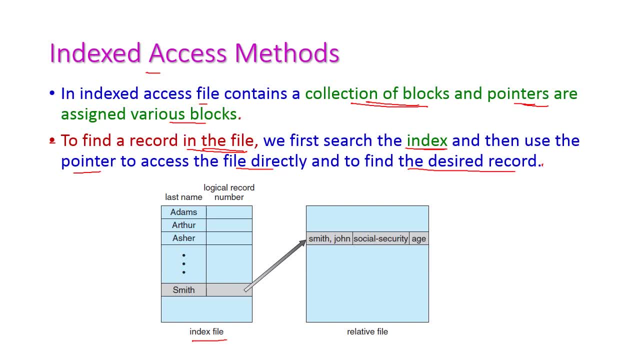 Okay, Here we are having a index file. In this index file, first the index is assigned to all the block. This is the index. Okay, And the corresponding pointer is there. Okay, Suppose I want to find a particular record. 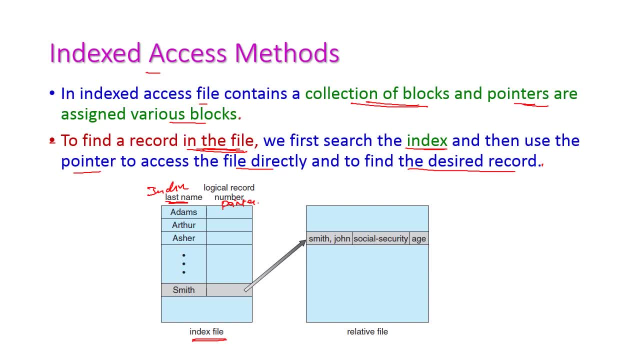 Then first I need to find this index, which is the index here? Smith is the index. Then by using this corresponding pointer, I can access the record in this relative file. Okay, Relative file contains the original data. Original data are records.